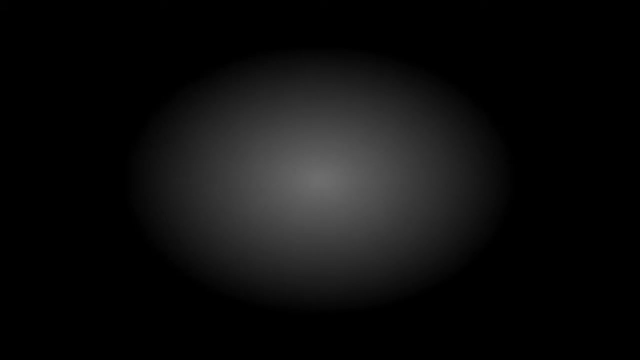 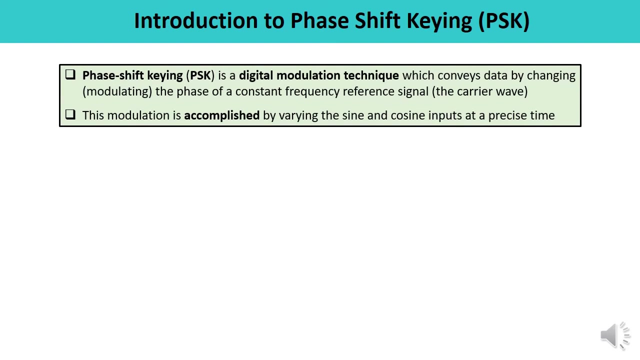 Let us begin. What is phase shift keying technique? What is PSK? So phase shift keying? it is a type of digital modulation techniques which conveys data by varying, by changing the phase of constant frequency reference signal, that is, the carrier wave, and this modulation is accomplished by varying the sine and cosine input at the precise time interval. 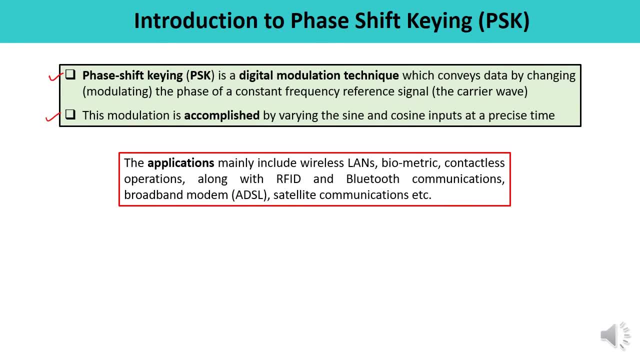 So the applications of PSKs are in a number of fields. It applications may include wireless LAN, biometric, contactless operations in RFIDs, Bluetooth communications, broadband modems, satellite communications and so many other applications are also there for the PSK. 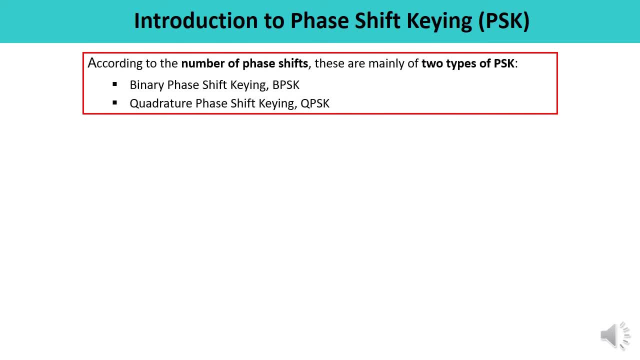 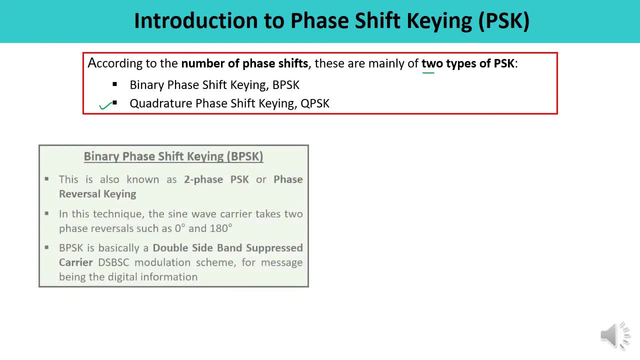 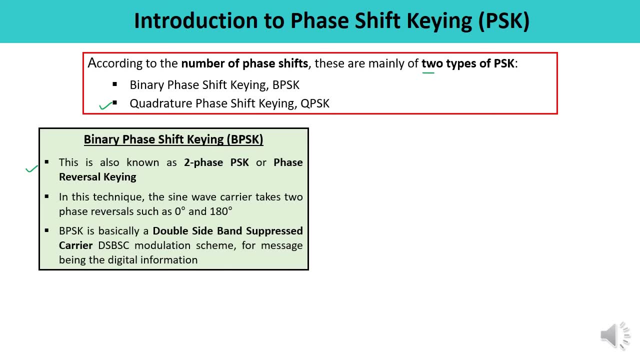 number of phase shifts accordingly, So BPSK. BPSK is also known as a two phase, PSK or phase reversal keying. In this technique, sine wave carriers take two phase reversals like 0 degree and 180 degree, and BPSK is basically a double sideband suppressed carrier, that is, DSBSC modulation scheme for message being the digital information and the second one which I am going to 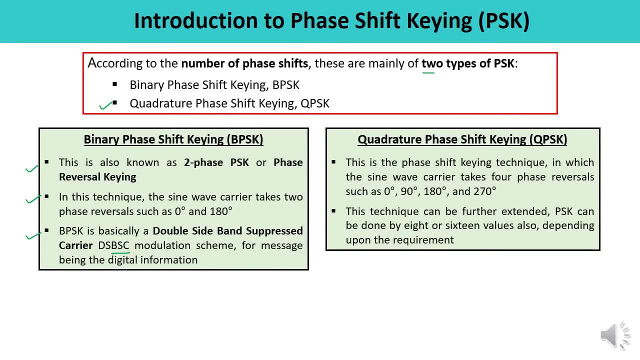 talk about in this particular video, that is, the quadrature phase shift keying. So quadrature phase shift keying is actually, in this particular case there are four variations, like in which sine wave carries carrier take four phase reversals, like 0 degree, 90 degree, 180 degree and 270 degree. and if this kind of technique are further extended, PSK can be done by using 8, 16 values accordingly. 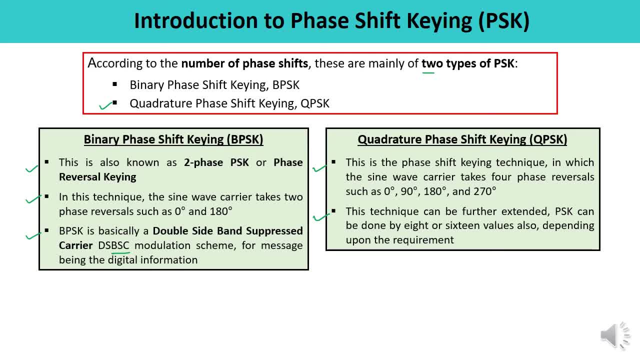 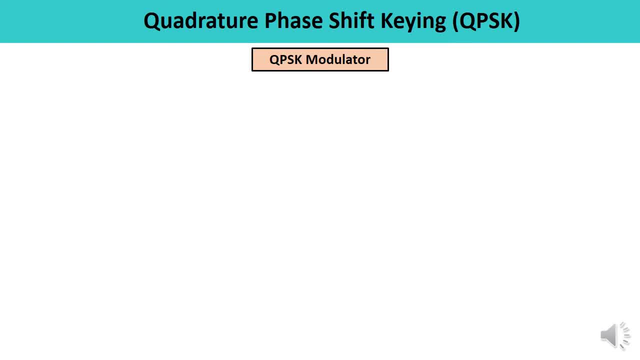 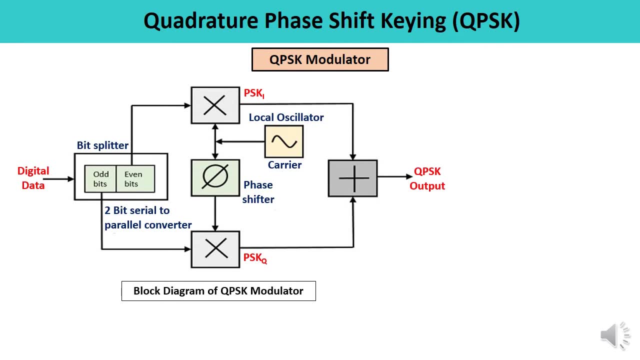 depending upon the requirement. So this has one advantage for the extension also. Now we are talking about the QPSK, which is the quadrature phase shift keying technique. This is the block diagram of QPSK modulator. but you must remember that QPSK, which is the 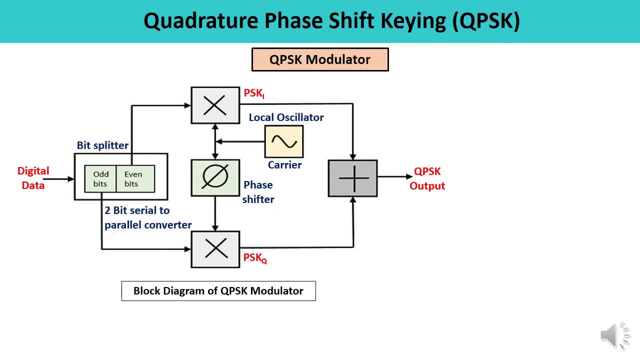 quadrature phase shift keying. that is the variation of BPSK right and it is also known as a double sideband suppressed carrier modulation scheme which sends two bits at a time. So this is the advantage in the case of the QPSK: It is capable to send two bits of digital information at a time. 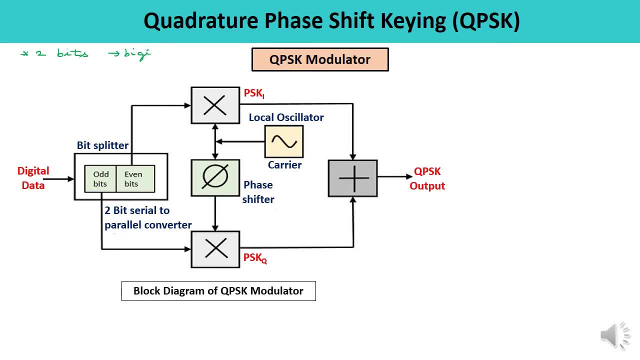 which is known as by jits right, and instead of conversion of the overall digital bits into a series of digital streams, it converts them into the bit pairs. So here the conversion is being done into the form of the bit pairs, and because of this it decreases the data bit rate. So here data bit rate is decreased, and this is decreased to. 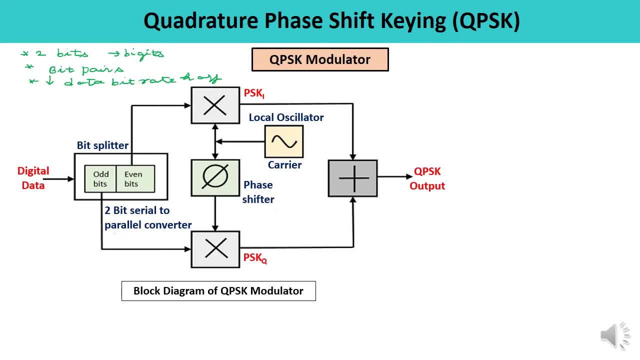 half because two bits are being transmitted at a time and because data bit rate is decreased to half. it means it allows space for the other users. Now let us discuss about the block diagrams. So in this block diagram you can observe the input is the digital data and at the output you will be. 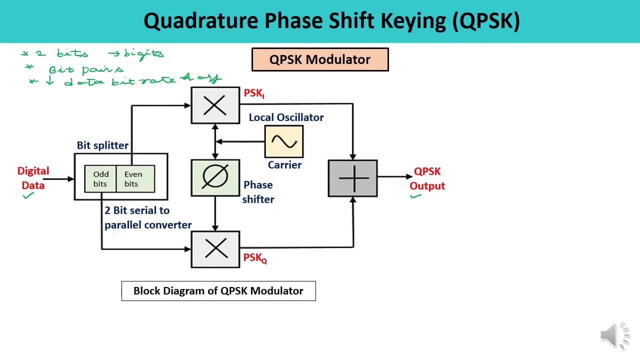 getting the QPSK output. There is a use of bit splitter, There is a phase shifter, carrier and adder or the summer circuit. So here what happens? the input data, which is the digital data which is available at the modulator input. So the message signal: even number of bits and odd number of bits. 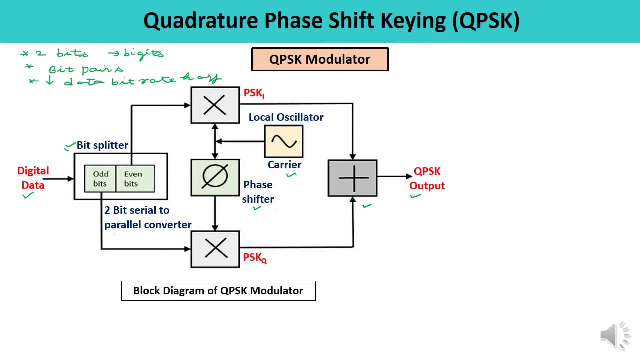 are separated by the bit splitter. Even number of bits like two, four means second bit, fourth bit, sixth bit, like on, and the odd number of bits like first, third and fifth. So these bits are separated out by the bit splitter, then they are multiplied by with the same carrier. Here you can observe, even number of bits are 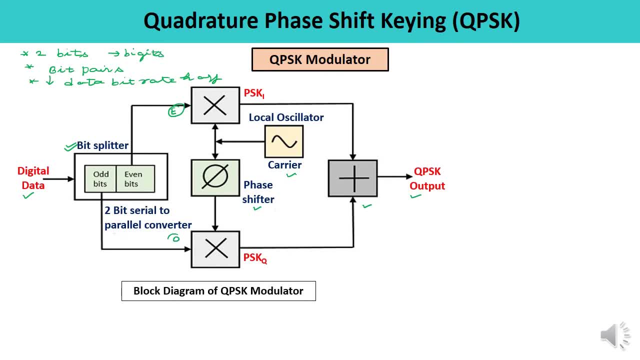 available at this particular point. odd number of bits are available at this point. Now they are multiplied with the carrier and this carrier is phase shifted: One carrier and number two carrier. So number two carrier will be 90 degree phase shifted. So what happened? So the bit splitted bits which are available now as a collection of even and odd. 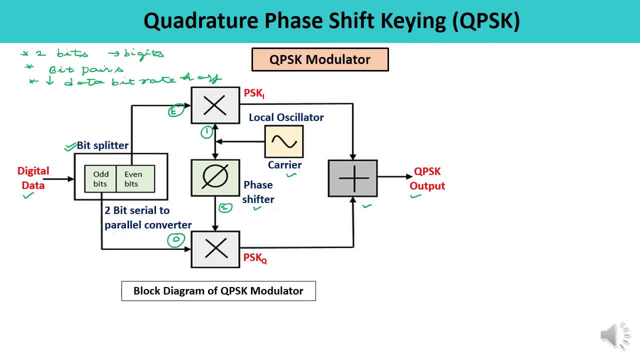 bits. they are multiplied with the same carrier to generate BPSK. with BPSK means phase shifting signal, which is known as a PSK- I means in phase- and PSK Q- that is the quadrature phase. So this is how the signal is being generated and the PSK Q signal that is anyhow, phase shifted. 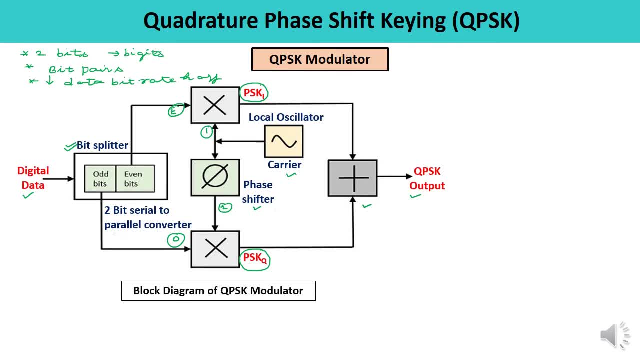 by 90 degree before it is being modulated. right, So you can observe PKSK signal. here the carrier is phase shifted by 90 degree- you have observed over here- and the two BPSK signals are then simply added means. here there is a adder: they are added together for the 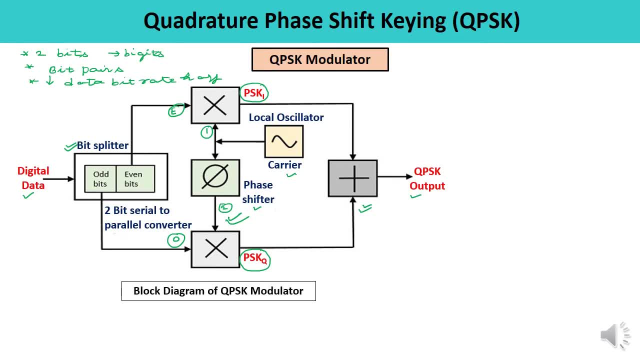 transmission Because they have the same carrier frequency. you have observed over here. there is the same carrier frequency and they occupy the same portion of the radio frequency spectrum. So the two sets of signals that would be mixed over here and the required 90 degree of phase, 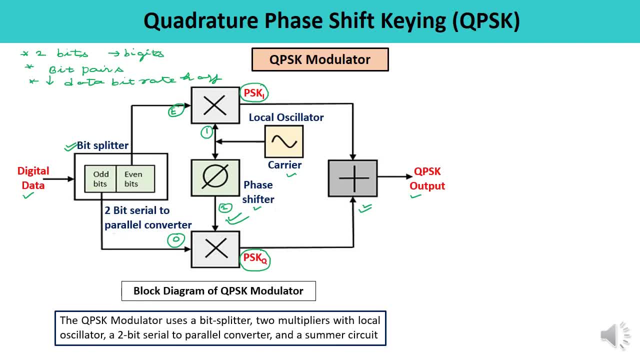 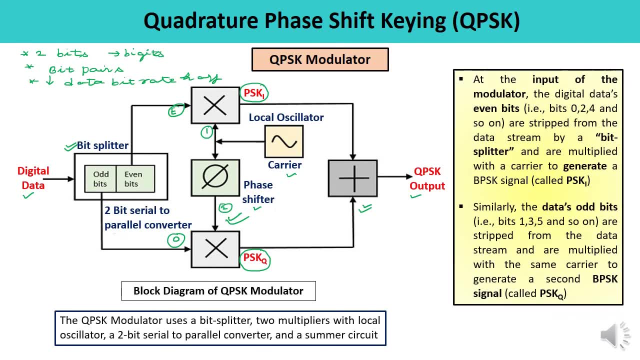 separation between the carriers that allows the sideband to be separated by the receiver by using phase discriminator. So this is how the overall entire operation is being performed and at the output we will be getting the QPSK signal. This is already I have explained to you and here you can observe. this is a carrier or. 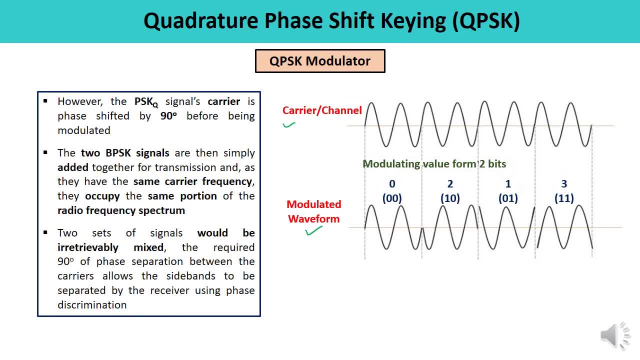 the channel and this is the modulated wave, and you can observe two bits are modulated at a time. that is why the data bit rate is being reduced. 0 means for 0 it is 00, for 2 it is 10, for 1 it is 0.. 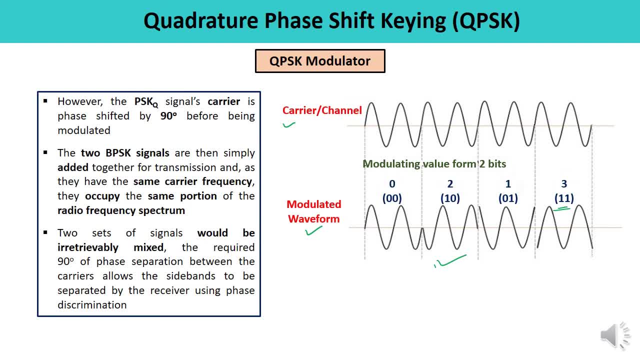 1 for 3: it is 0.. 1 for 3: it is 0.. 1 for 4: it is 0.. 1 for 5: it is 0.. 1 for 6: it is 0.. 1 for 7: it is 0.. 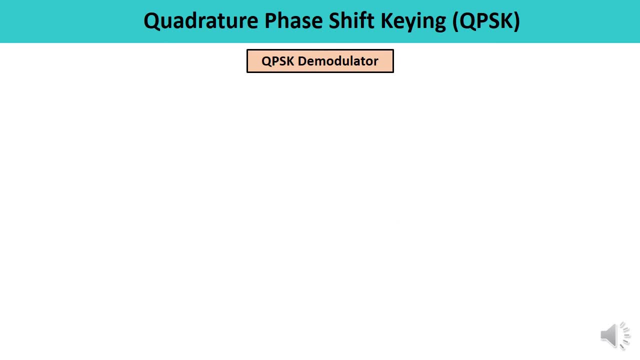 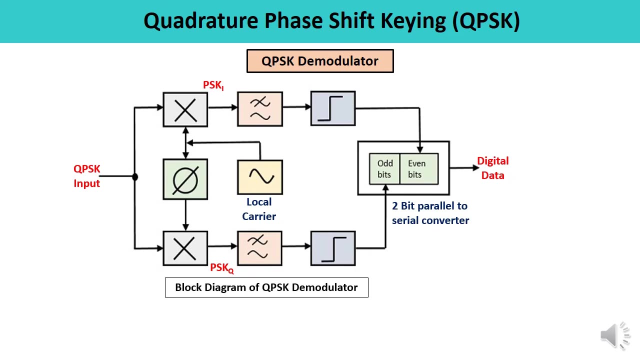 1 for 8, it is 0.. 1 for 11.. So this is how you can represent it. this is the QPSK waveform. Now let's talk about the QPSK demodulator. So this is the block diagram of the QPSK demodulator. 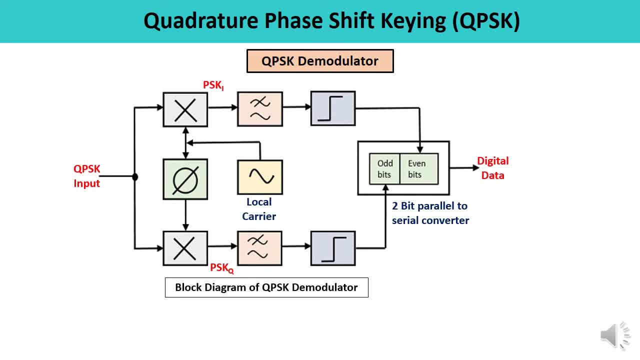 You can see the QPSK demodulator. it uses two product demodulator circuit. here two product demodulator circuits are there. there are two local oscillators. you can see mixers, two integrators right and two bit. parallel to serial converter means even an odd number of bits will be mixed. 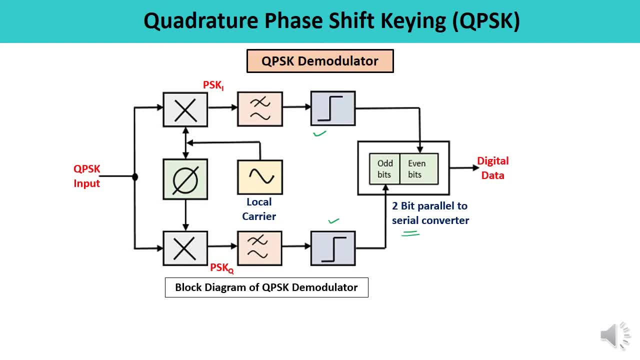 together and then they will be processed. So here the two product detectors at the input of the demodulator. here the input is what the input is, the QPSK input, and at the output we require the digital data which is to be separated out. so the two product detector at the input of this demodulator. they simultaneously. 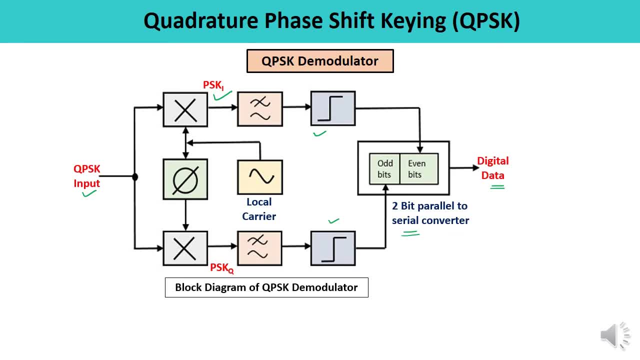 demodulate the two BPSK signal. the two BPSK signals are what PSK I and Q, which are in phase, and the quadrature phase means overall circuit arrangement. you must be able to explain with the help of each and every block right. 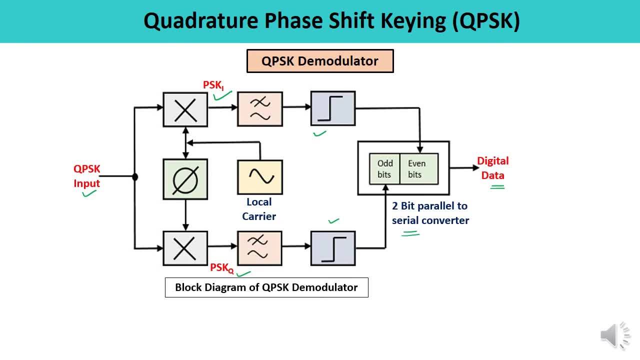 So this pair basically simultaneously recovers the pair of bits in the original data and the two signals are cleaned up using a comparator or some other signal conditioners. Then the bits are put back in the order by using this two bit parallel to serial converter. 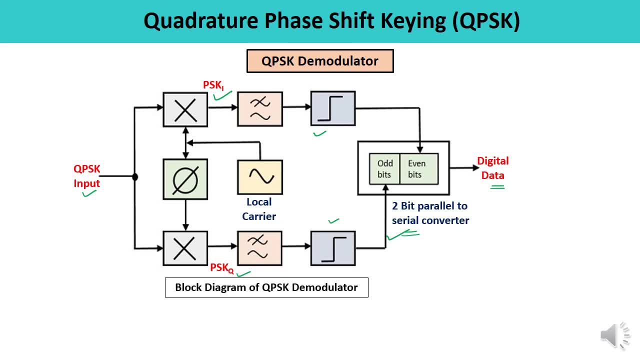 So each detector picks out only one of BPSK signal, not the both. only one of the BPSK signal means it may be a in phase or quadrature phase right. So recovery of message signal will be optimum if the transmitted and the local carrier are. 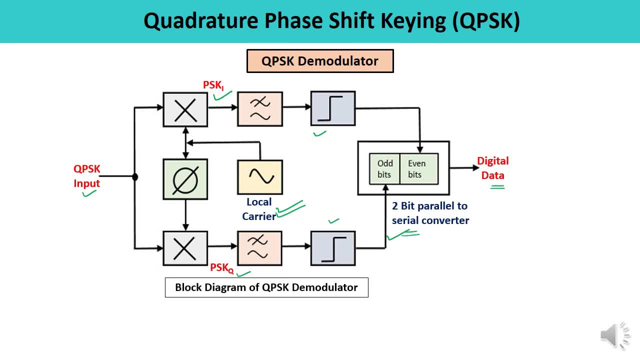 in phase with each other. So the local carrier and the transmitted signal are in phase. So the local carrier and the transmitted signal are in phase. So the local carrier and the transmitted signal are in phase. will be in phase. then it will be very easy. but the recovered message is attenuated if the two 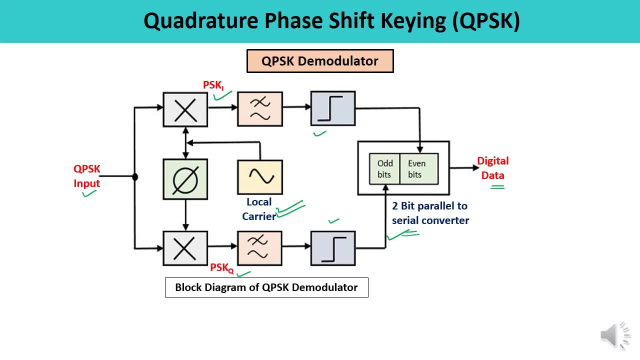 carriers are not exactly in phase and when the recovered carrier is attenuated means there is a phase error. right, it means the amplitude of the recovered message is zero in that particular case. so, product detector, they share the carrier but one of them is phase shifted right and once the phase of the local carrier for one of the product detector it matches with the. 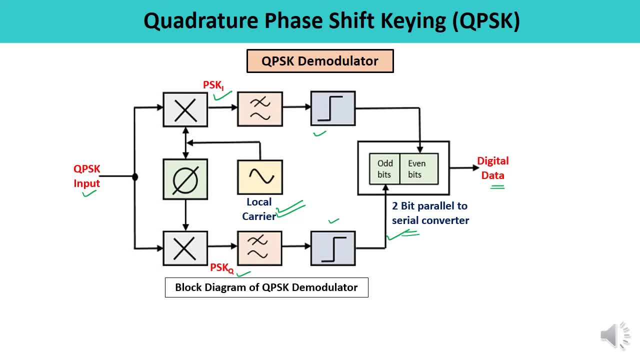 phase of the transmission carrier of one of bpsk signal. it means there is automatically a 90 degree phase error in between the detector's local carrier and the transmission carrier of other bpsk signal. therefore, the detector recovers the data on the bpsk signal which is matched. 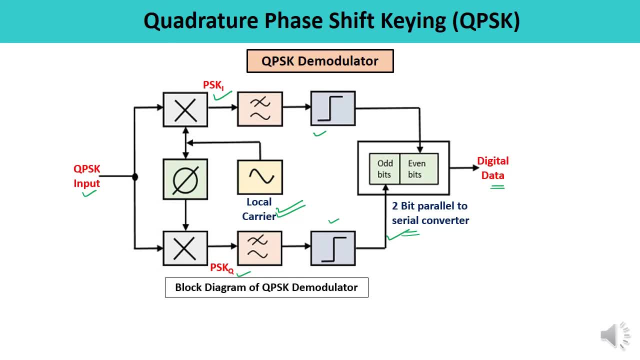 and and reject the other bpsk signals. so overall process is very simple, like it is: first again multiplied with the local carrier, then being integrated by and bypassing the filter and then by just using do two bit parallel to serial converter at the output we will be able to get: 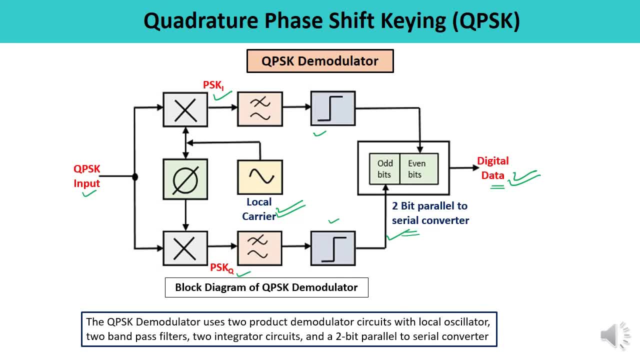 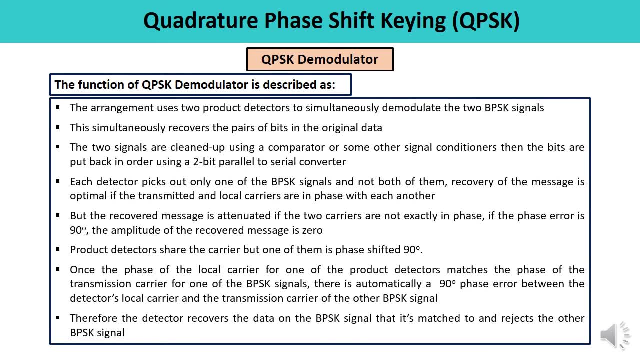 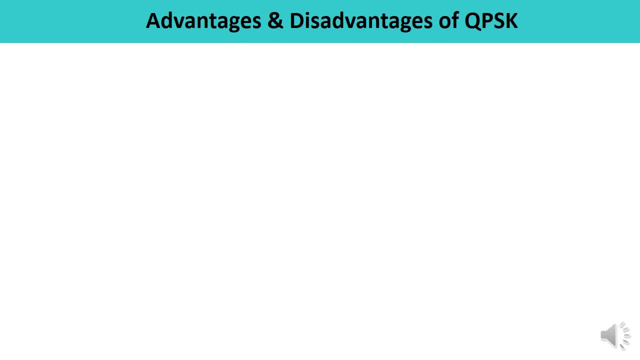 the digital data back. so this is how you can explain the qpsk demodulator. the function of qpsk demodulator i have listed out over here. i have already discussed this. now in the last, let us talk about the advantages and disadvantages of qpsk. the advantages are: it provides very good noise. 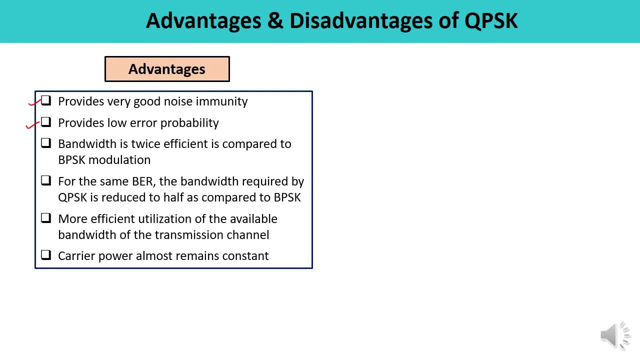 immunity provides low error probability. bandwidth is twice efficient in comparison to the bpsk modulation and for same bit error rate, the bandwidth required by qpsk that is reduced to half in comparison to the bpsk. it is more efficient means utilization of available bandwidth is being done in a more efficient way and carrier power almost remains constant. these